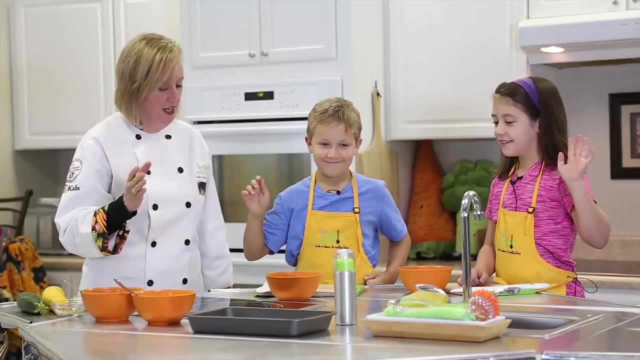 writing with. I don't know which hand I'm writing with. I don't know which hand I'm writing with, right, I'm glad you guys know. Okay, this is the hand that you are actually going to grip the knife with, Alright, and we'll say: you guys want to use like a bicycle. 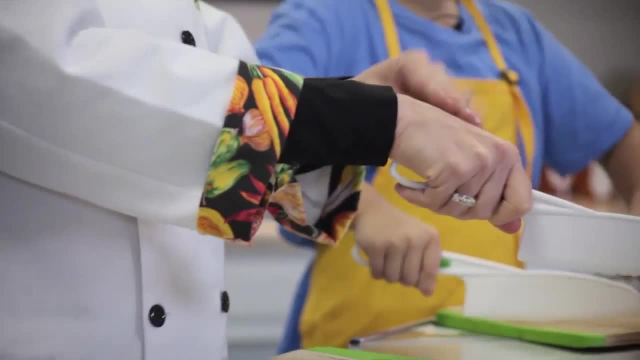 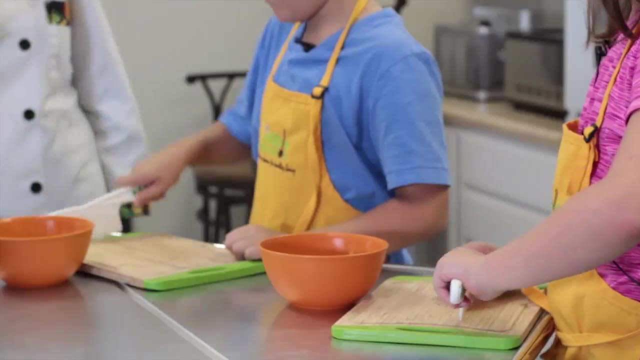 grip, a motorcycle grip. We want the top part of our hand up. If you guys are doing it like this, it's called carpal tunnel syndrome when you're 30, alright, So we're going to have the top part of our hand up- Brilliant. Now, before we start to wheel. the way is this: 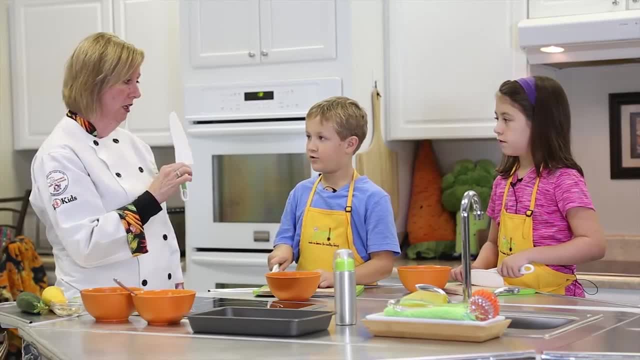 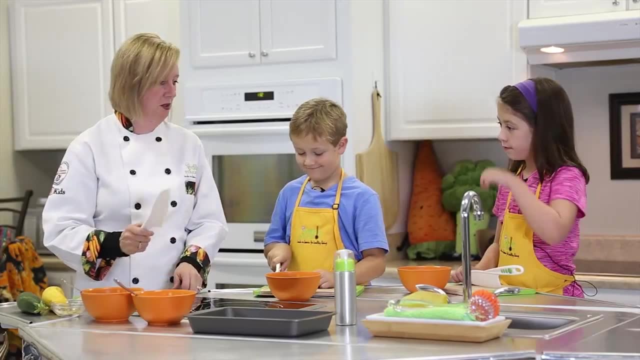 a tool or a toy Tool Tool. Excellent answer, Right answer. If it was a toy, we'd be out in the jungle gyms, right, But it is a tool, which means we're not goofing around today, Alright, so. 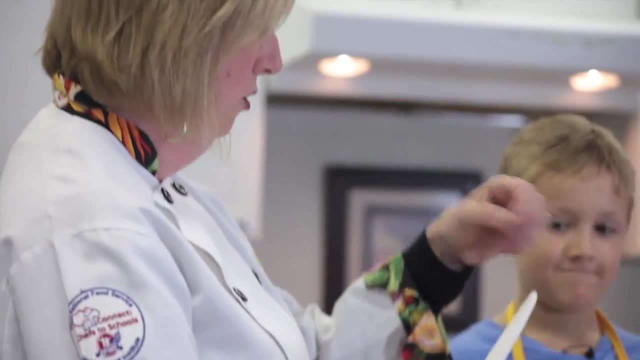 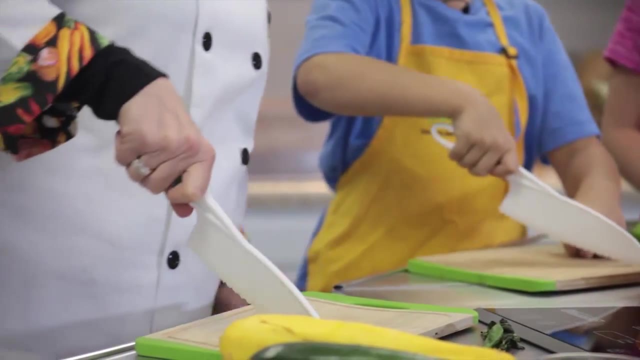 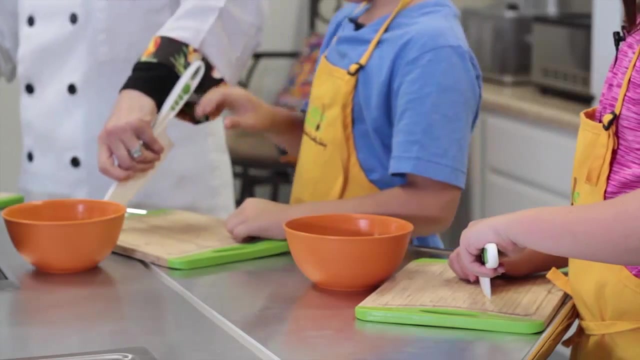 the next thing you want to do is put a little pretend super glue on the end of your knives. Alright, Glue, glue. Where's your glue, Nicholas? We're going to glue those knives right to the board, And we kind of want it perpendicular here, so we're going to glue. Claire is lefty. 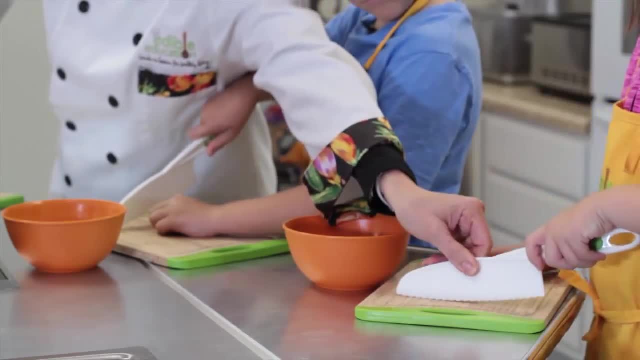 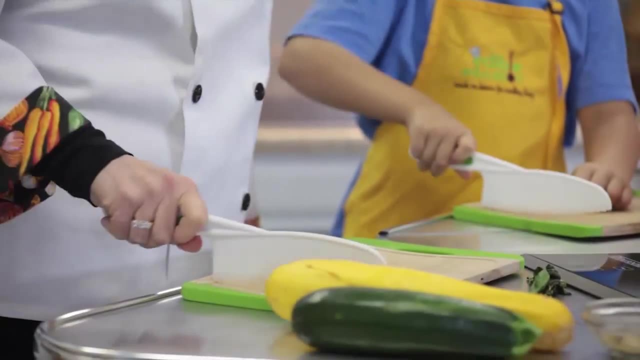 so she's gluing it this way: Boom chakalaka, right like that. Okay, now you guys see how the knife is a curved motion. Okay, that means here we are all day long. Okay, Miss Claire. 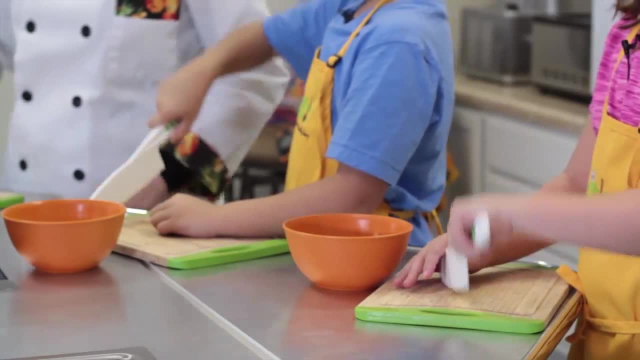 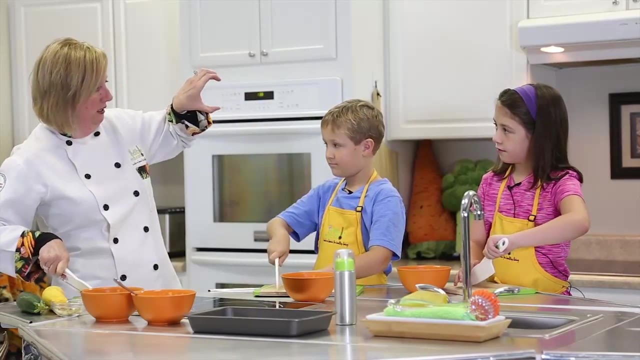 she's done this a couple times before. but what you want to do is just have a rocking motion. Hey, wait a second. We got this hand over here. What are we doing with this hand? Okay, we make the letter. What letter is it? 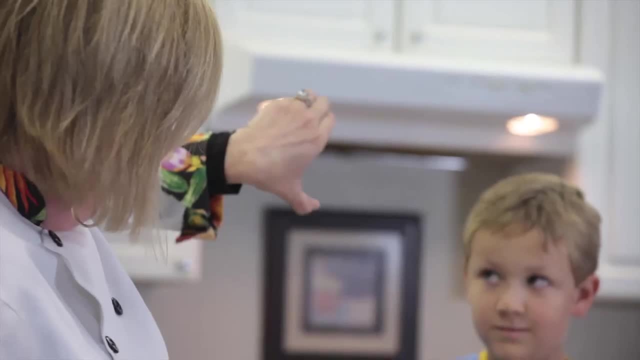 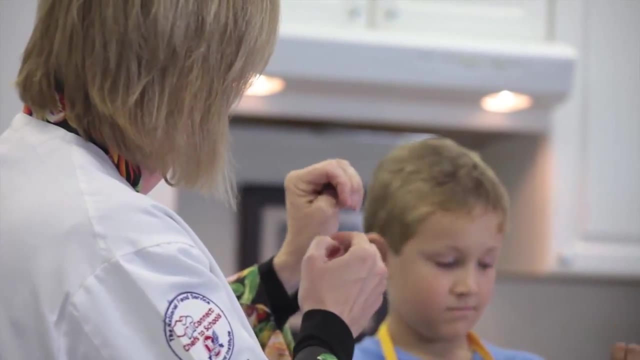 Two, What letter is it? C, C. Okay, so you guys hold up the hand that you're not writing with and you're going to put your thumb and tuck it over, So we call that putting our bear in the cave. I kind of dig. 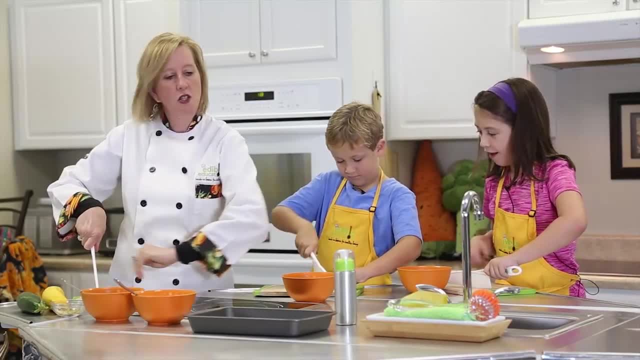 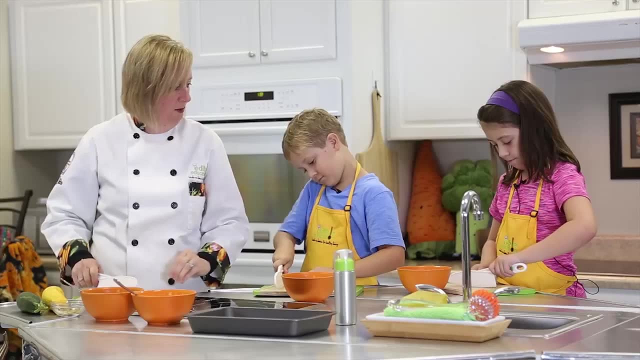 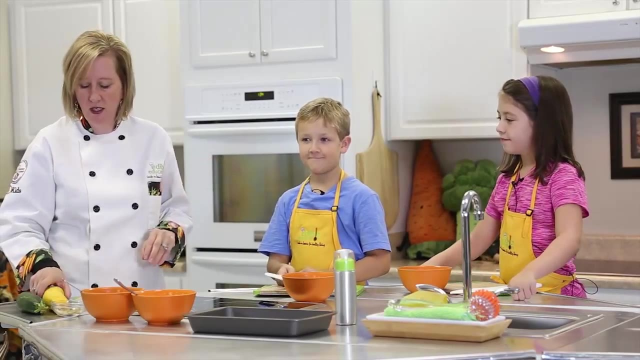 my fingernails into the food. So let's practice Chicken arms out and we're going to push the food to the knife. Good job, good job, Push Okay. you guys ready to do it with real food? Okay, This is the best easy, simple recipe. 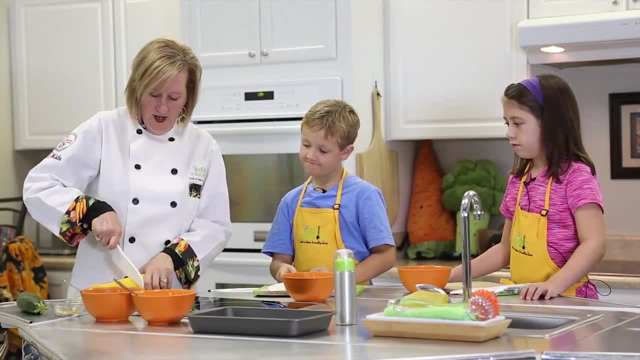 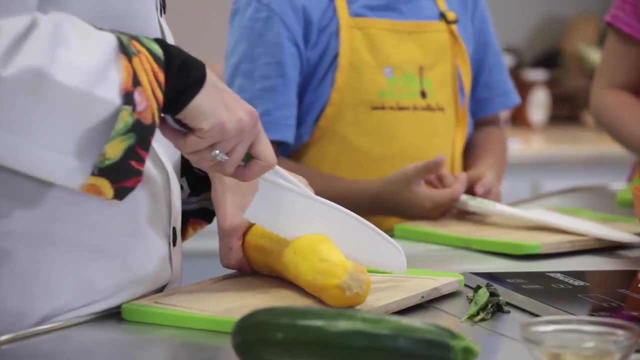 all right, Are we cutting this in half? Let's cut this in half. Okay, if you're cutting something that's a little bit too hard to cut with your knives, like this, like we said, with bear in the cave here, you could do flat hand on top- All right, there we go there.